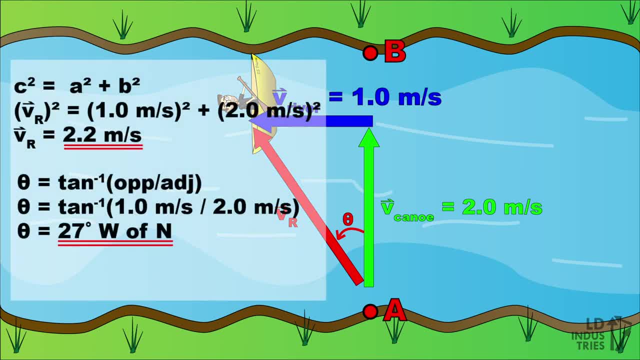 We can even work out how fast we'll be moving. We can use the Pythagorean formula to get the magnitude of the resultant, which works out to 2.2 meters per second, and the inverse tan ratio to get the angle, which will be 27 degrees west of north. 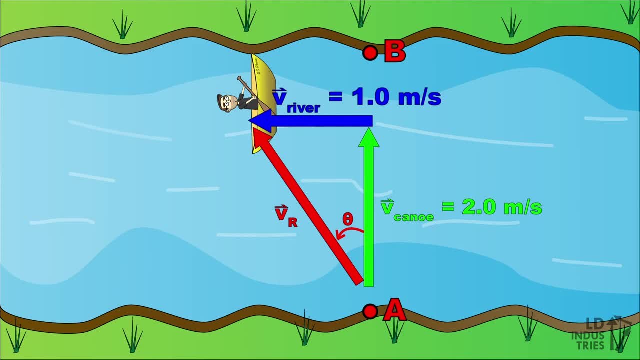 So how far down river did we end up? For this we need the width of the river. Let's say it takes 10 meters to travel from point A to point B. We can add that vertical or y-displacement vector to our diagram. 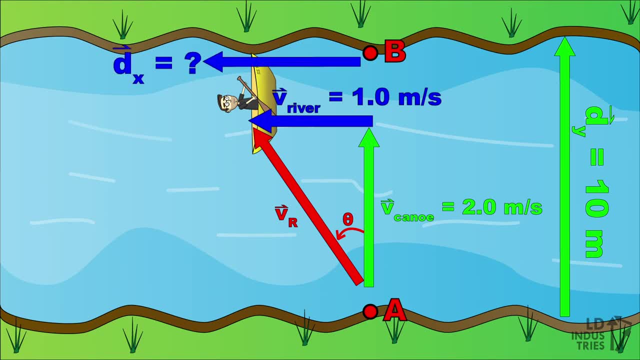 Here's the vector that represents the displacement of the canoe going downstream, the horizontal or x-displacement. So how are we going to figure that dx out? Well, we can model the motion of the canoe with a uniform motion formula: v equals d over t. 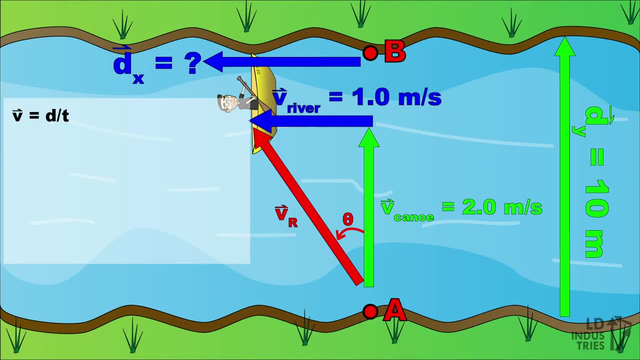 This makes sense, since the canoe is not accelerating while it's in the river. Substituting into this formula is a lot trickier, though. We can put in 10 meters for the displacement, I guess. but what velocity should go in? 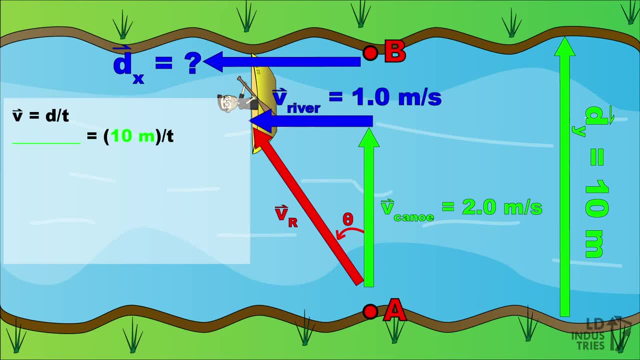 There are three different choices here. There's a key idea here that helps you work this out. When you're working with kinematics formulas, you need to substitute in x-vectors with other x-vectors and y-vectors with other y-vectors. 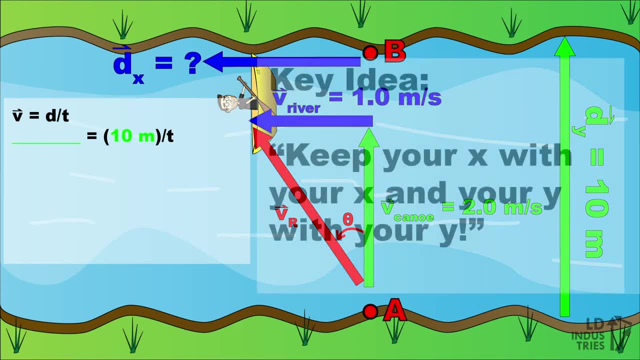 Or, as I often say in class: keep your x with your x and your y with your y. This means that if you substitute in a y-displacement, like 10 meters, you have to also sub in a y-displacement. 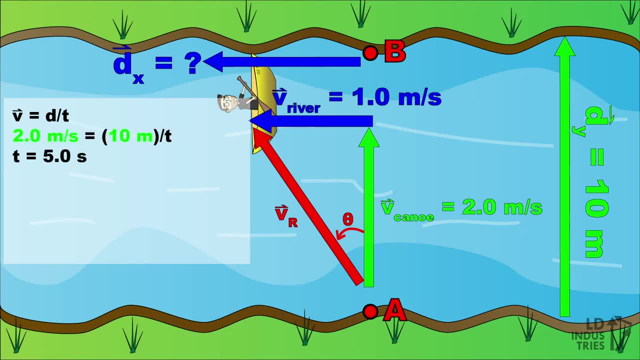 This means that if you substitute in a y-displacement like 10 meters, you have to also sub in a y-velocity, in this case 2 meters per second. That will allow us to calculate a time of 5 seconds. 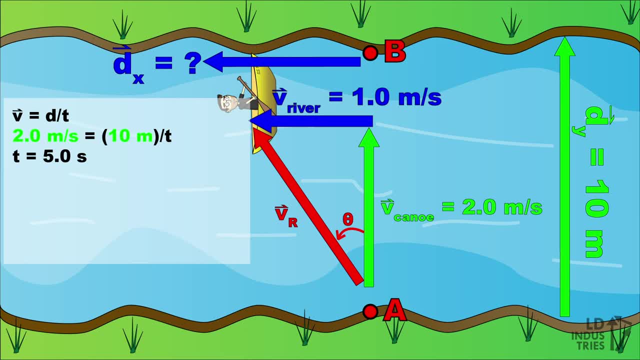 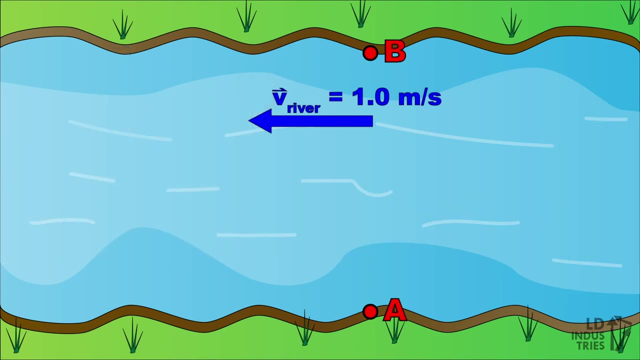 which is how long the canoe is in the water for. After we know the time, we can do a second uniform motion calculation for the x-direction. This time we'll use the x-velocity of 1 meter per second, along with the time to get the x-displacement of 5 meters. 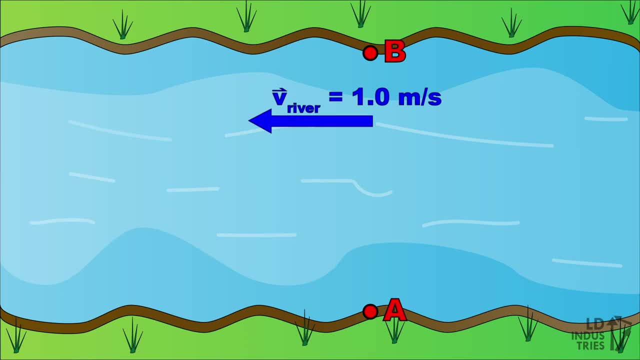 Lastly, what if we wanted to go from point A to point B exactly without drifting any? How could we make that happen? Well, we would need to paddle our canoe into the current, actually aim ourselves a bit to the east to counteract the motion of the water moving to the west.